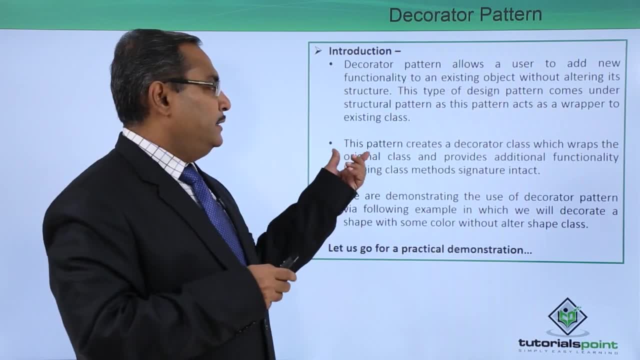 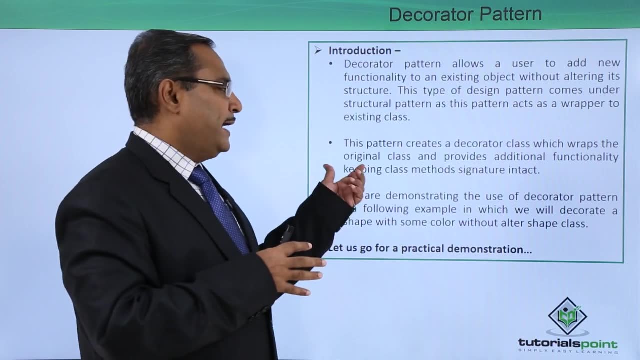 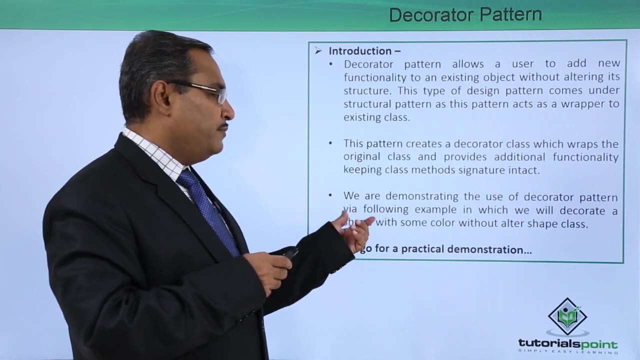 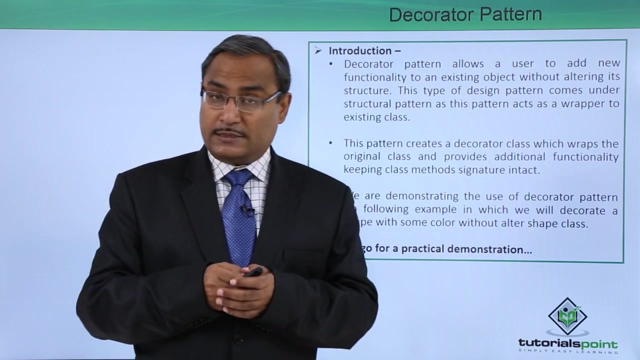 wrapper to the existing class. This pattern creates a decorator class which wraps the original class and provides additional functionalities and keeping the class methods signature intact. We are demonstrating the use of decorator pattern by a following example, in which we will decorate a shape with some color without altering the shape class itself. So we are 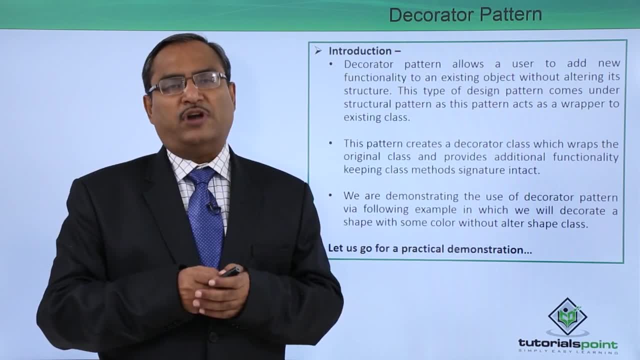 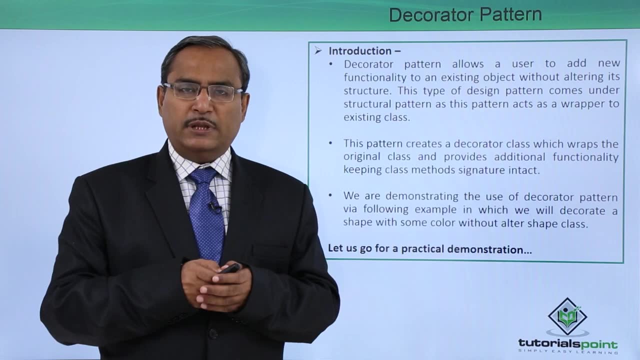 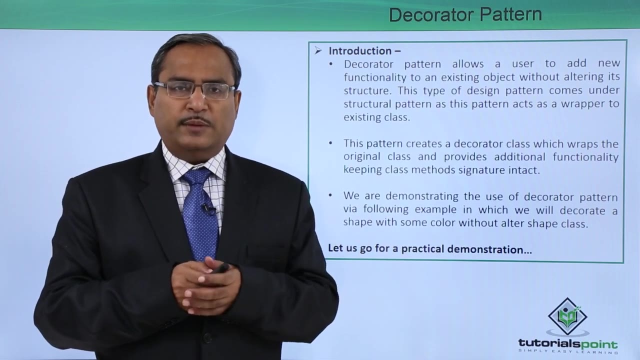 adding more functionalities to a class without changing the class structure. So that is the basic theme behind this decorator design pattern. So let us go for one practical example using Java, where we will be showing that how this decorator design pattern can be implemented. So here is the demonstration for you. In this session, we are discussing 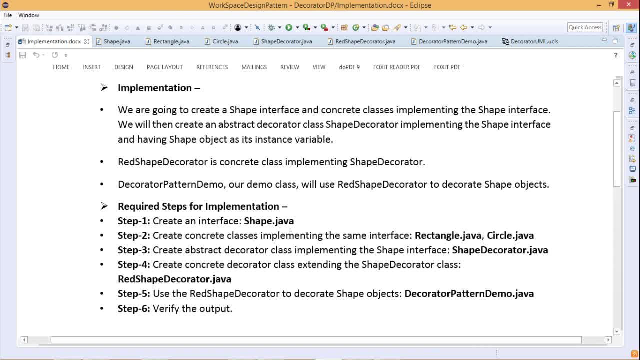 the implementation of decorator design pattern using Java coding. So here we are going to create one shape interface and the concrete class which will be implementing this shape interface, And we will then create an abstract decorator class. The name of the class will be shape. 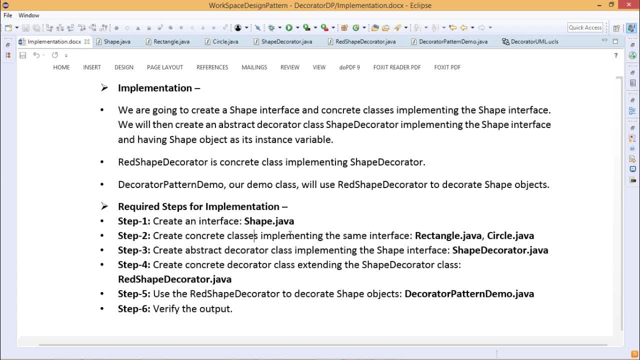 decorator implementing the shape interface and having shape object as its instance. variable Red shape decorator is concrete class implementing shape decorator And this particular decorator pattern demo will be our demo class, where we will be producing our outputs and which will use the red shape decorator to decorate shape objects. So to have the better clarity, 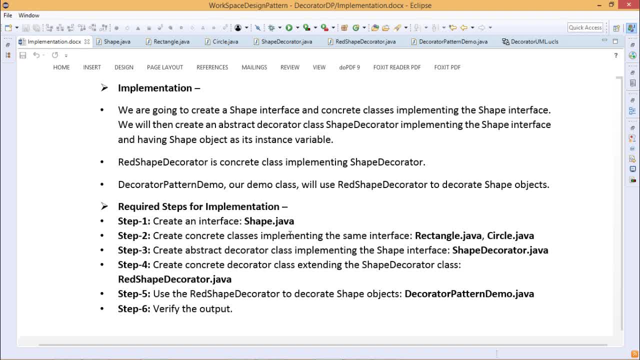 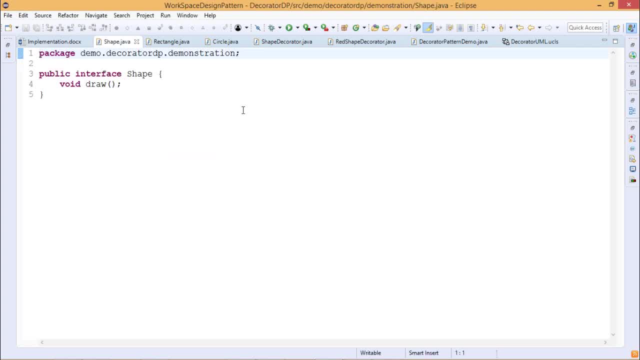 on this concept, On this planning. let us go step by step. At first, we shall create one shapejava, that is, one Java interface. So this is our Java interface. we are getting So public interface, shape. So name of the interface is shape, and it is having only one unimplemented method. 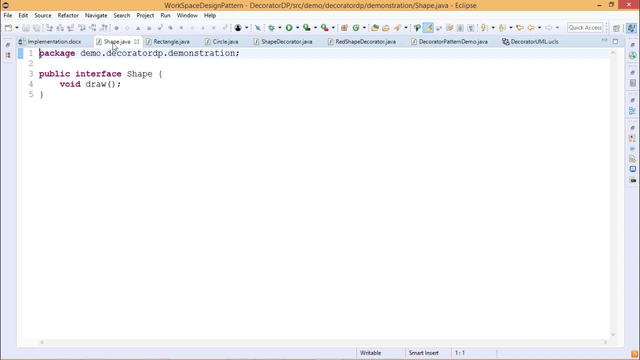 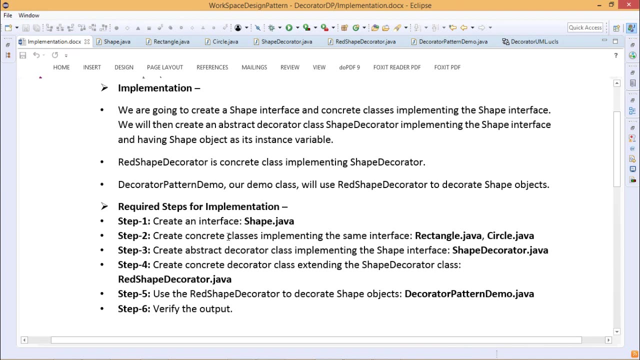 that is a draw which returns void. So we have defined one shape interface which is having only one method unimplemented. that is draw. Next one is about create concrete classes implementing the same interface. So we will be going for concrete classes which implement. 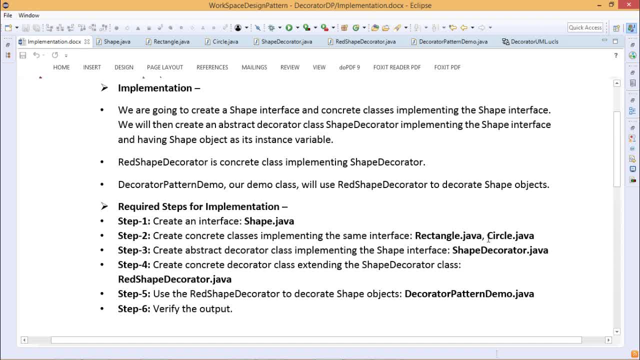 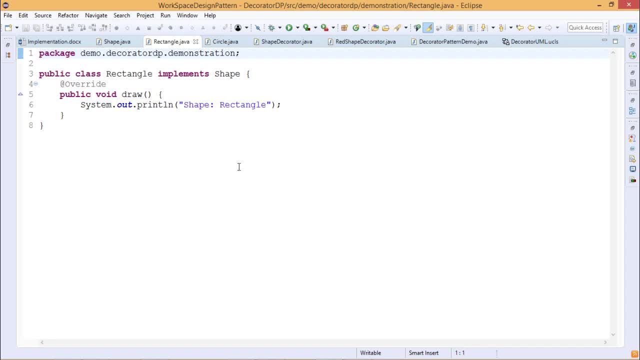 interface shapejava, So let they be rectanglejava and circlejava. So this our rectanglejava, which is implementing the shape and also overatning the draw method. So these respective string is getting printed if I execute the draw method, And similarly for the circle, this particular. 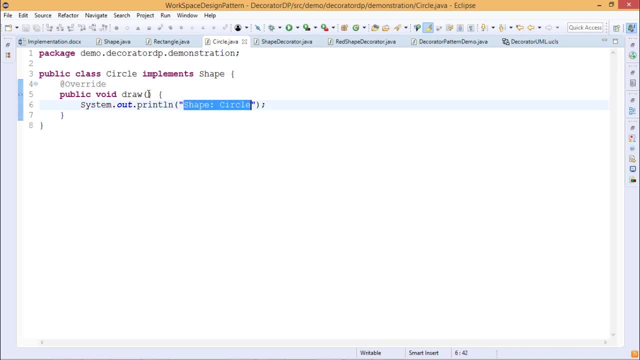 shape colon circle will be printed if we execute this draw method. So this circle is nothing but a class. the shape interface rectangle is also nothing but a class implementing the shape interface, and both of them have implemented the code against the draw method. so i think now this concept is 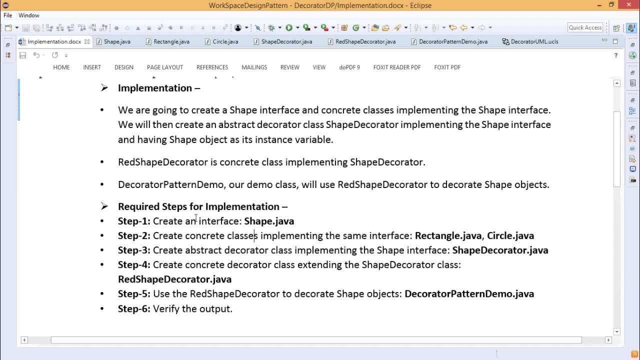 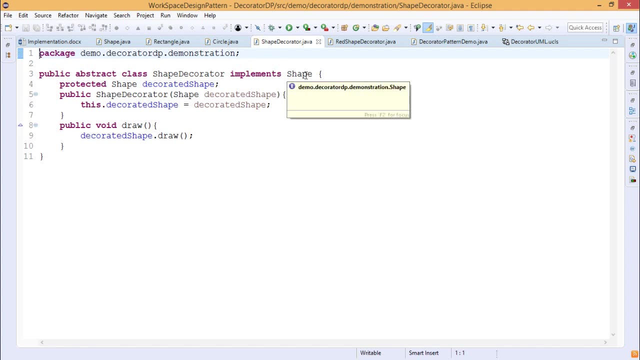 clear up to this level. okay, now we shall go for the create abstract decorator class implementing the shape interface, and name of the class will be shape decorator dot java. so let us come to this shape decorator dot java which implement shape interface. as it implements shape interface, so the draw method must be overwritten, must be defined here, so public void draw. that is a. 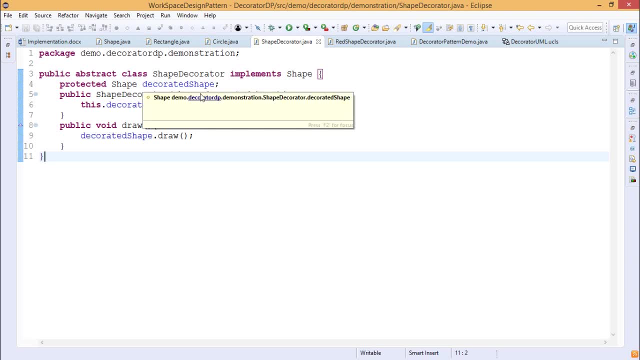 decorated shape, dot draw. so decorated shape is nothing but one instance variable under the class decorator, shape decorator, so protected. so it is, remember this one. it is under the scope protected, so can be inherited also if i require so protected shape, decorated shape, we are having. and And then public decorator, shape decorator, it is nothing but the constructor. 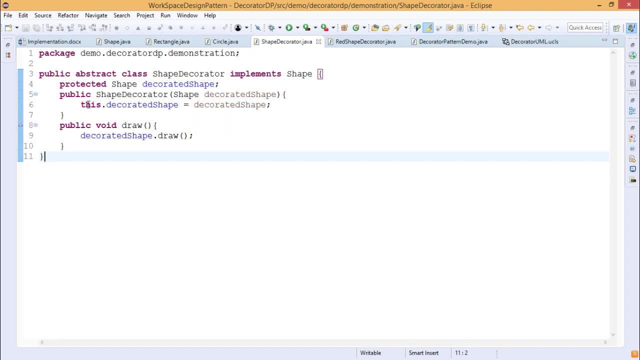 which takes this shape object as input argument, inputs parameter, And this dot decorated shape will be instantiated, will be initialized with this decorated shape. There is a shape object And draw method we have overwritten here, which will just execute the decorated shape. 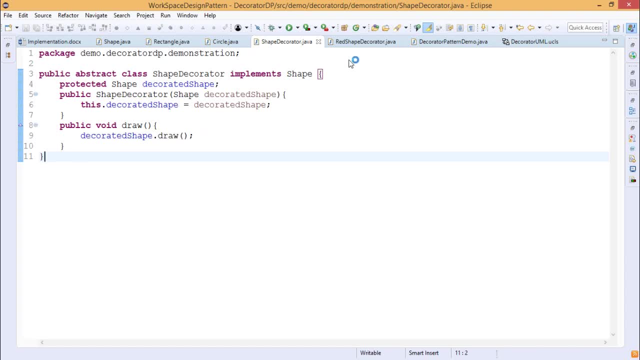 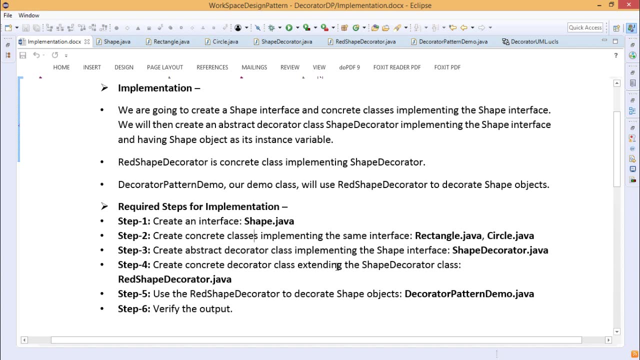 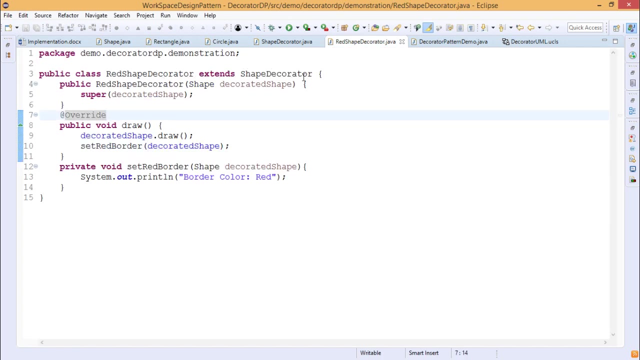 That is the instance: variable decorated shape dot draw. Next one we are going for. that is our red shape. So create concrete decorator class extending the shape decorator class. So that is our red shape decorator. So in case of red shape decorator which extends the shape decorator, 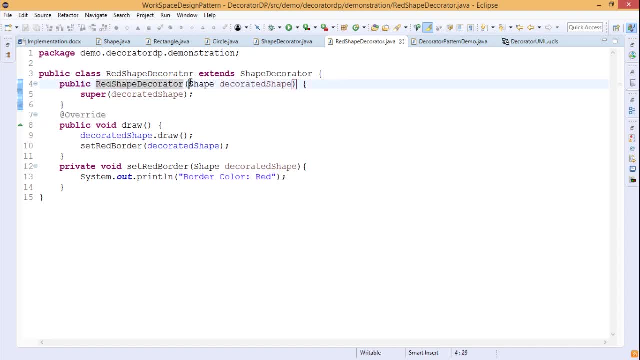 So red shape decorator is a constructor here which is having one shape object as input parameter And it is calling the base class constructor. It is calling the base class constructor using the keyword super. So this decorated shape is the object shape class. 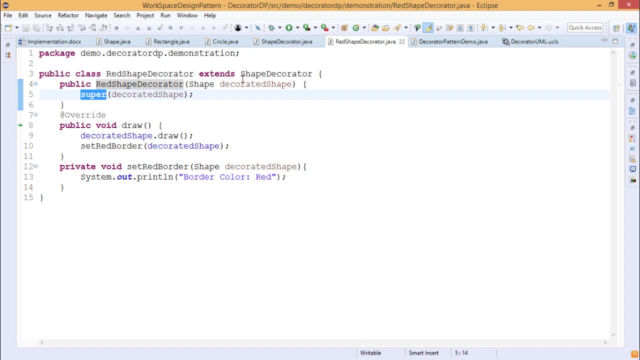 Object has been passed as the input argument. So here the base class is the shape decorator, Its constructor. that means this particular constructor will go on executing. So this particular decorated shape, this particular decorated shape which has been passed as input argument. 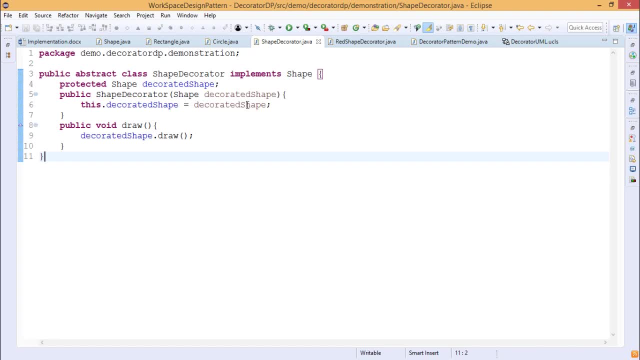 will be assigned to this decorated shape And this dot decorated shape is equal to decorated shape. So now it will go to instantiate the instance variable. Next, we are having this draw method, So there is a overriding, the draw method. So here we are writing: decorated shape- dot draw. 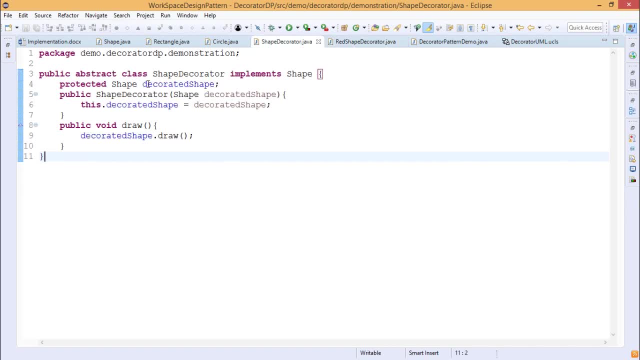 So that is the decorated shape. From here this decorated shape has got inherited Because this particular red shape decorator class is inheriting the shape decorator. So that is why decorated shape dot draw, So this particular method will be called. 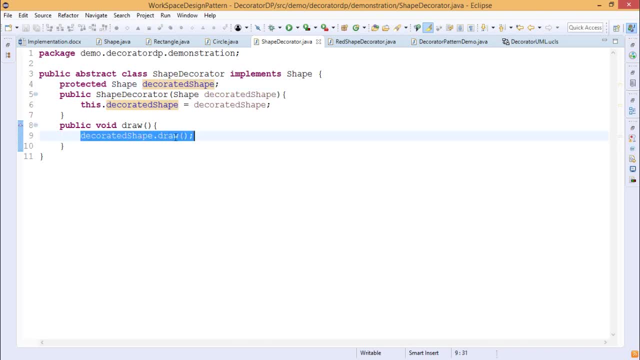 And, as a result of that, this particular method will be called ultimately. So you see, it is calling the shape, So that means the shape, So this particular method will be called here. So now, along with that, we are going for set. 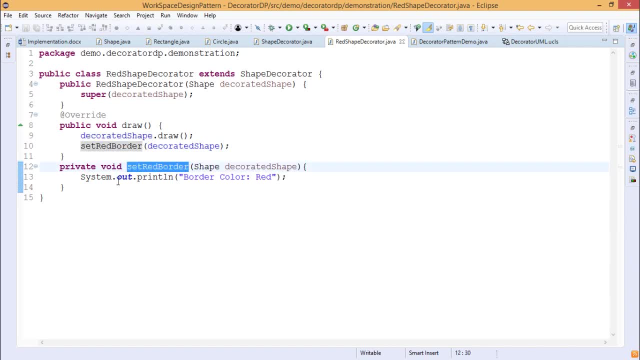 Red border, So one method which has been locally defined here as the member method here. So here we are passing this decorated shape, So now this set red border. So shape, decorated shape, And then system dot outer println border. color colon: red. 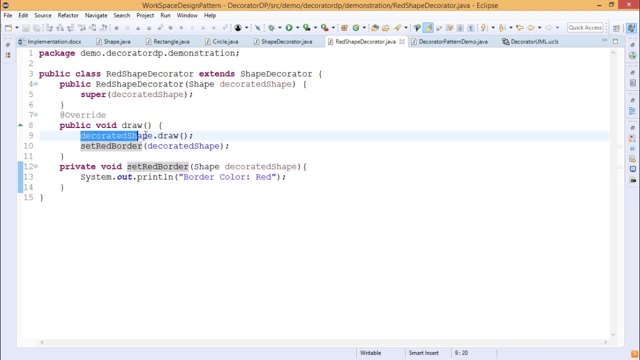 So we are going for the decoration here, So this decorated shape dot draw the method will be called Along with that. this particular method has been called And this method is printing the string. There is a border color: colon red. 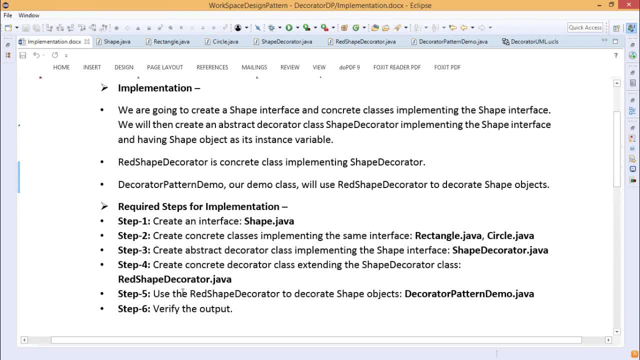 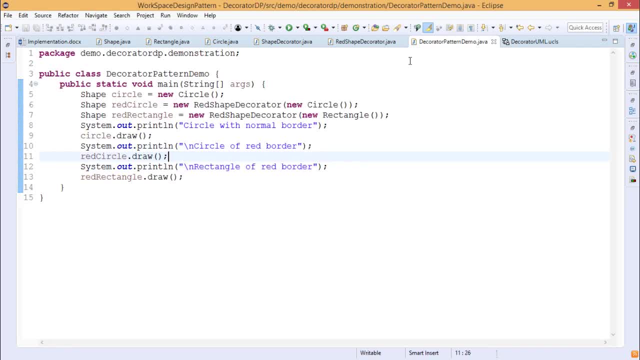 So now we are going for the last class, That is, the use the red shape decorator to decorate the shape object. So: decorator pattern demo dot java and verify the output. So this is the decorator pattern demo dot java. So here we have defined one circle class. 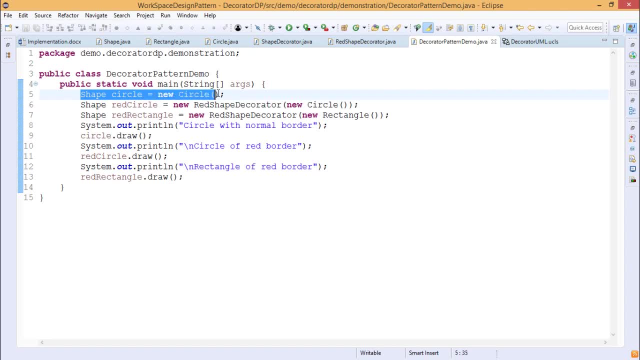 Circle object under the interface shape is going to be new circle. So ultimately we are going to create one circle class object here. So shape red circle and shape red. So now it is equal to new red shape decorator, new circle. And it is new red shape decorator, new rectangle. 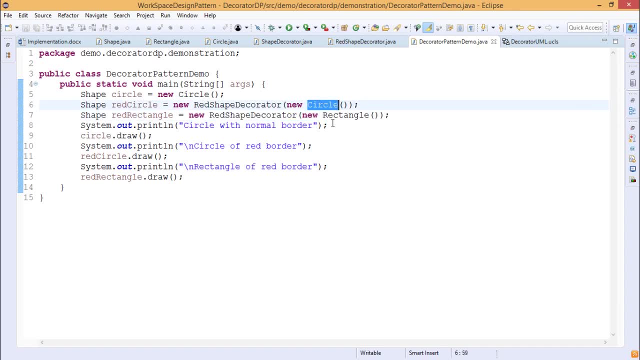 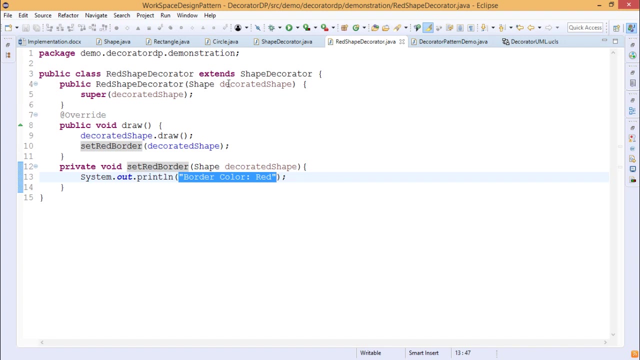 So now, in the first case we are passing one circle class object as input argument. Here we are passing the rectangle class object as input argument to this constructor. red shape decorator. So if you come to this red shape decorator, you can easily find that its constructor is taking shape class object as input argument. 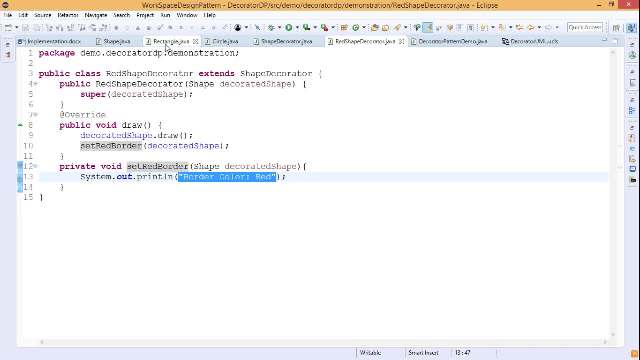 So shape. So shape is not a class. Shape is nothing but an interface, And this rectangle dot java will be the implementing class of the shape interface. So as a result of that, whenever this shape object can be passed, So there you can also pass our rectangle class object or circle class object. 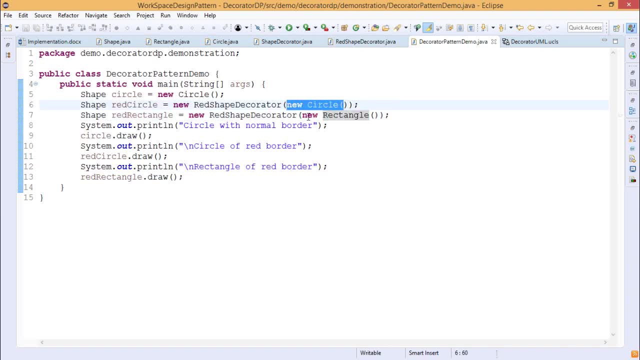 So that is why here you can find that we have passed that circle class object and also the rectangle class object in the next time. So now, if you go for the circle dot draw, If you go for the red circle dot draw, If you go for the 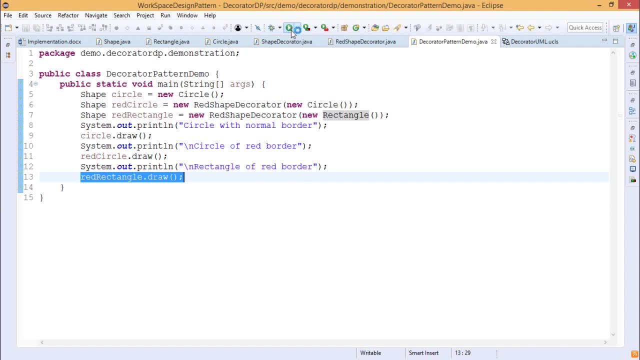 Red rectangle, dot draw will be getting the output like this: So these outputs we are getting. So full code is there, Output is also there, You can go for a match. So now, at first, we are having this: This is a shape. circle is equal to new circle. 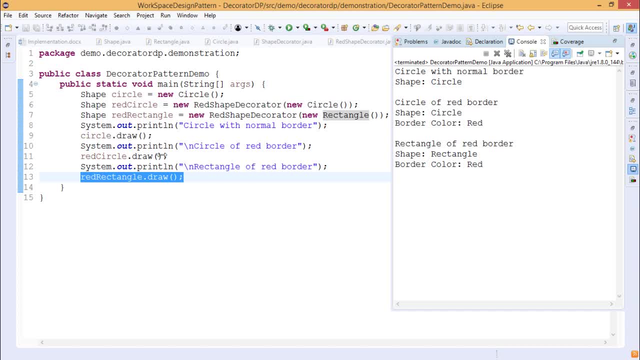 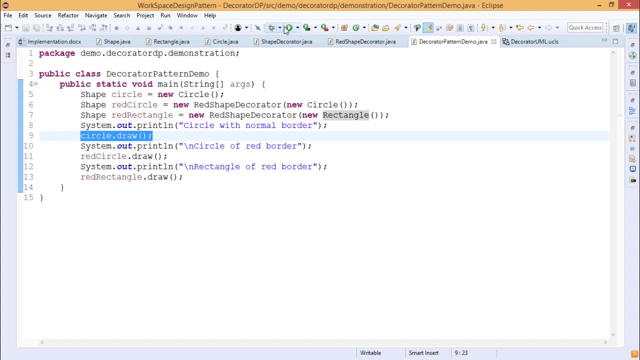 So it is a mere circle class object. So whenever I am printing, Whenever I am printing this particular string from this draw method, There is a circle dot draw. We are getting this output, something like this: We are getting this output. 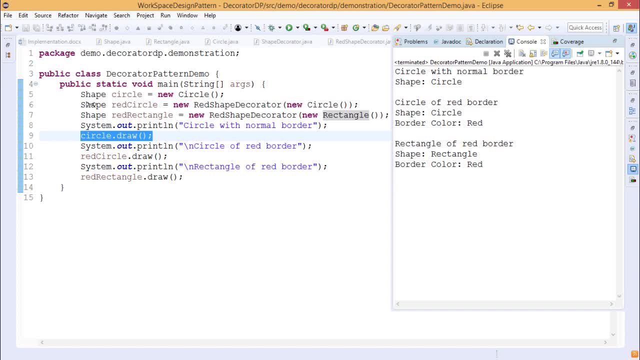 There is a shape colon circle, But here you see, this shape red circle is equal to new red shape decorator, New circle. So whenever we are printing this red circle dot draw, Not only shape colon circle will be printed But along with that the border color colon red will be also printed. 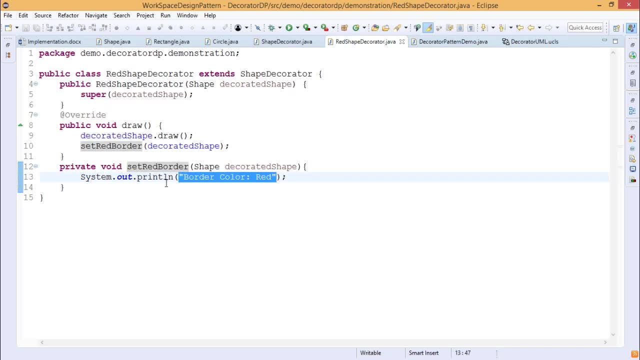 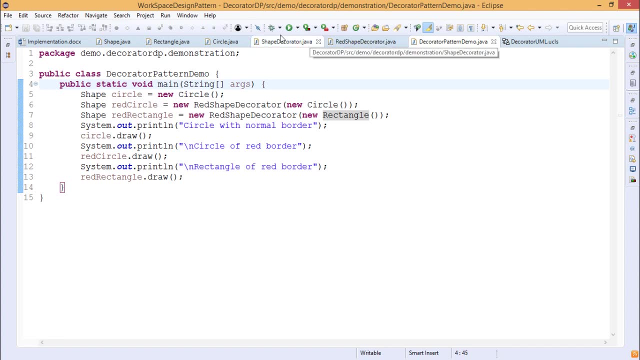 So you can get it here. So not only this one, So also the border color red will be also printed. So at first it will be called, and then this particular method will be called here. So in this way we are getting the next output. 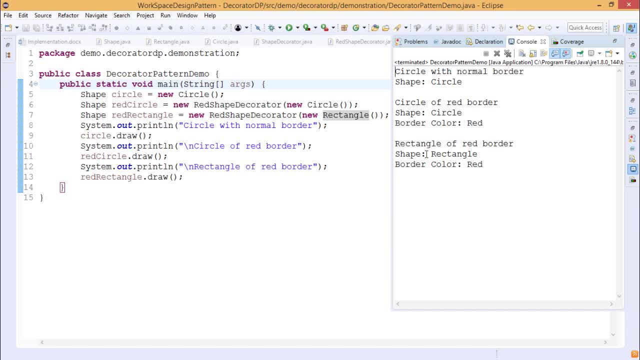 That is a rectangle, So rectangle of the red border. and then we are having this shape: colon rectangle and the border color colon red. So rectangle of the red border and then red rectangle dot draw. So it is just printing this line and also this line. there is a border color colon red. 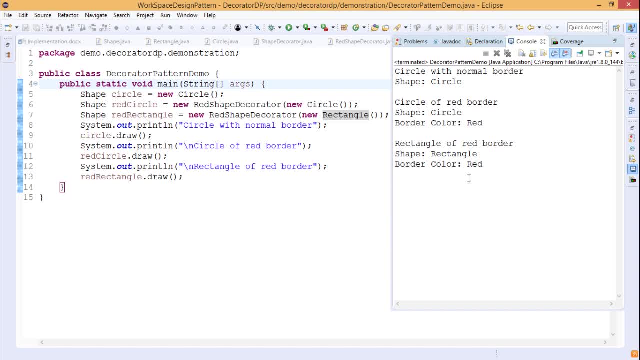 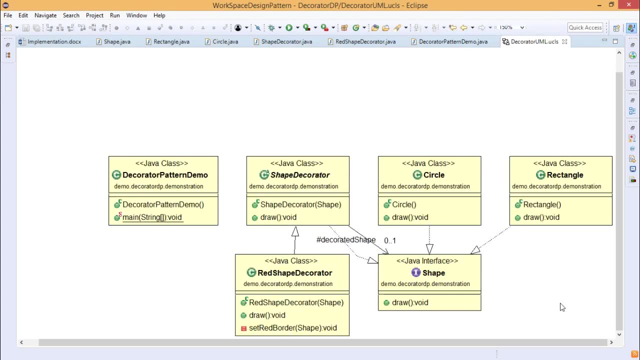 So in this way you are getting this idea how this decorator design pattern can get implemented using our Java code. So let us go for the class diagram for the same. So here we are having the class diagram. So shape is nothing but one interface. 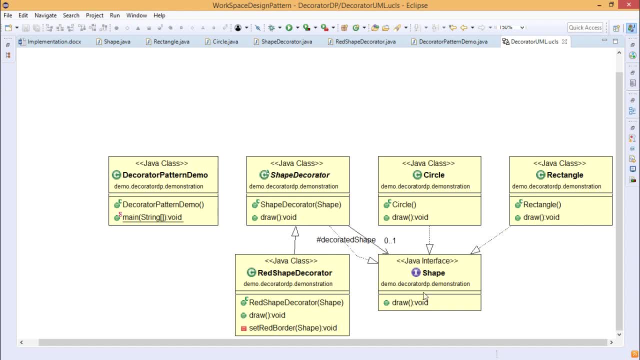 Having only one method unimplemented, that is, our draw, This rectangle and the class circle. These two are the implementing Java classes, So they are implementing the shape. So that is why they are having this draw method overwritten there. And this is our shape decorator.